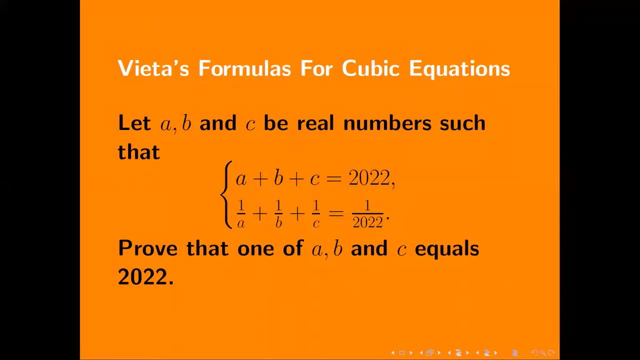 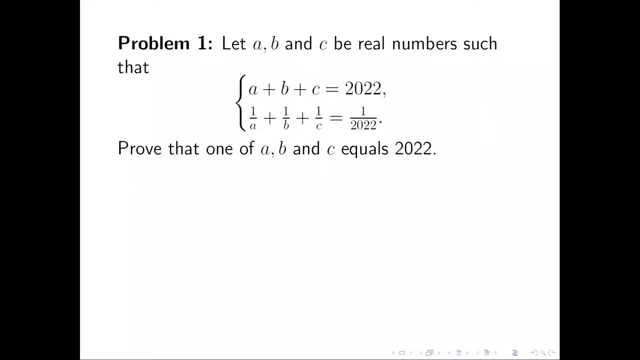 Veritas formulas are suitable for solving equations with symmetric or cyclic variables. In this video, I am going to present some applications of Veritas formulas for cubic equations. We are going to solve two problems. The first one: let A, B and C be real numbers, such 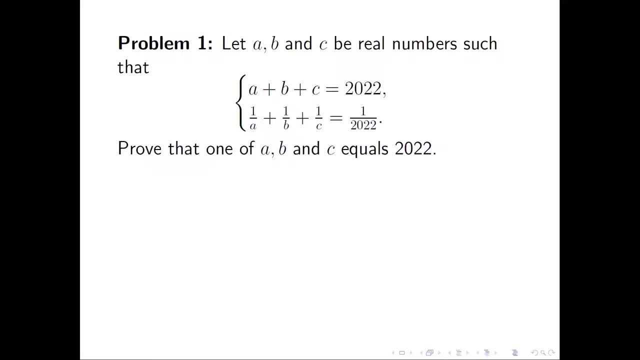 that the sum of the three numbers is 2022, and the sum of the reciprocal of the numbers is 1 over 2022.. Prove that one of the numbers, A, B or C- equals 2022.. The second one: we want to solve the systems of equations in three variables. 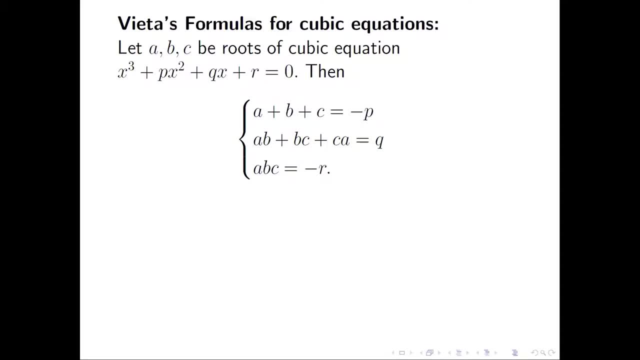 We start with a brief description of the theorem. We start with a brief description of the theorem. We start with a brief description of Vieta's formula for cubic equations. Let A, B, C be roots of cubic equation. X, cubed plus PX, squared plus QX plus R equals zero. 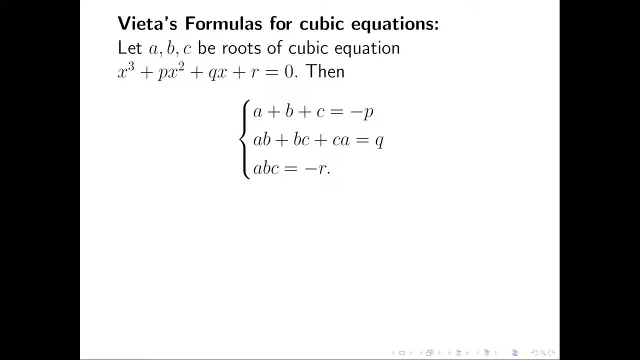 Then the sum of the three roots A plus B plus C is negative P, And AB plus BC plus DA equals Q and the product ABC equals negative R. A simple proof: By zero-root theorem, the polynomial can be rewritten as X minus A. 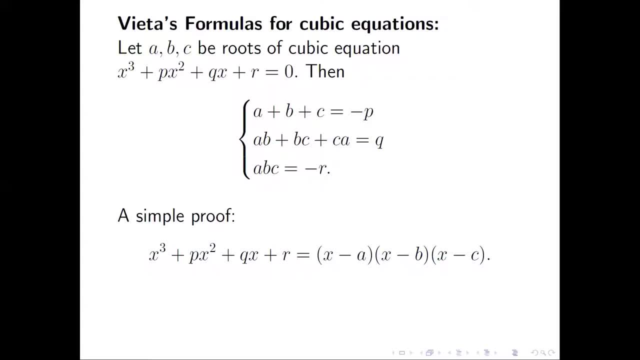 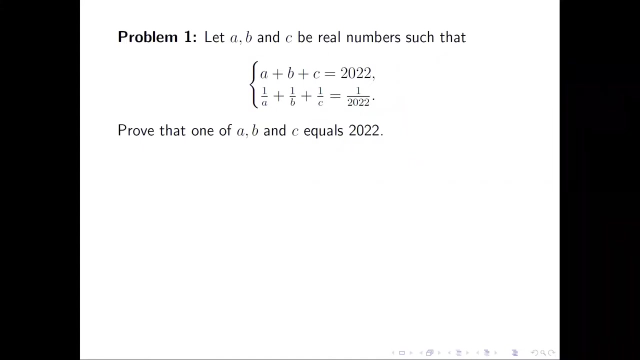 the first root, times X minus B, times X minus C, the other couple of roots, If we expand the right-hand side, combine the like terms and compare the coefficient for both sides, where Vieta's formula are then established. Now let's solve the first problem. 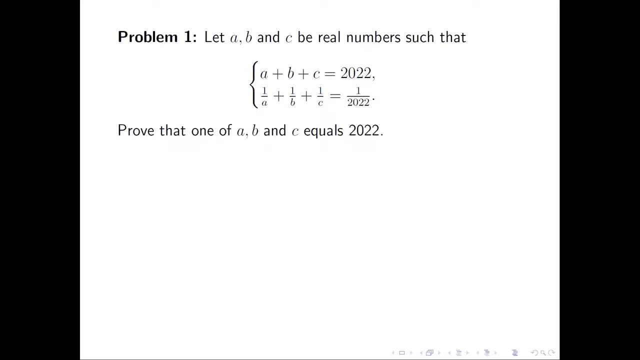 We have three variables with two equations. There are infinitely many solutions, but for all these solutions, one of the variables has to be 2022.. From the second equality we multiply all the denominators A, B, C and 2022. 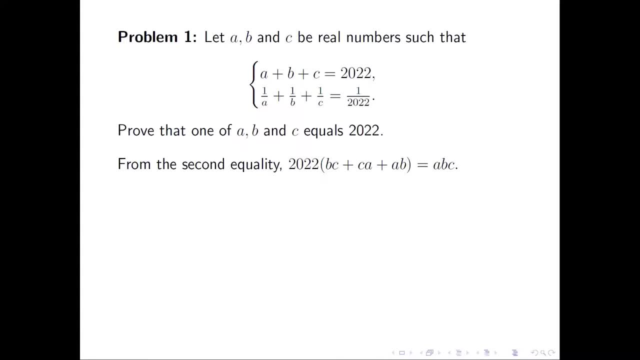 We multiply all the denominators A, B, C and 2022.. We have a 2022 times BC, plus CA plus AB equals ABC. Now we see all the three elements in Vieta's formula. First, we have A plus B plus C, which is 2022. 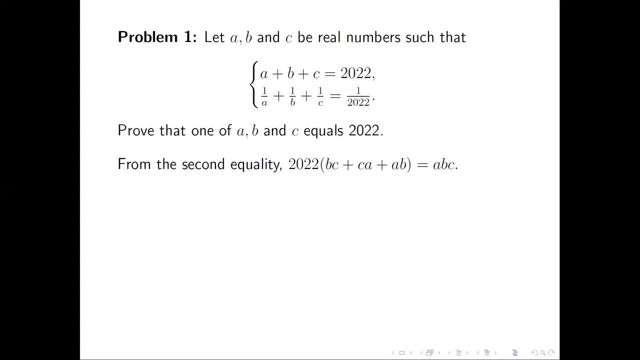 We also see a relation between the second and the third element in the Vieta's formula. The second element, BC plus CA plus AB, times AC is correct. times 2022 equals the third element, a, b, c. Let's a b plus b, c plus c, a equals q. 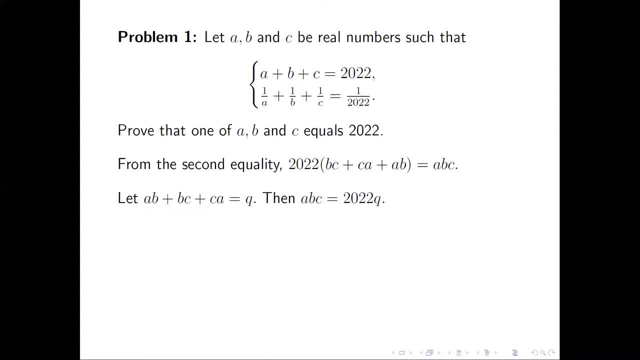 Then a, b, c is 2022 times q. From Vieta's formulas for cubic equations: a, b and c are the roots of the cubic equation x. cubed minus 2022. x squared plus qx minus 2022, cube equals zero. 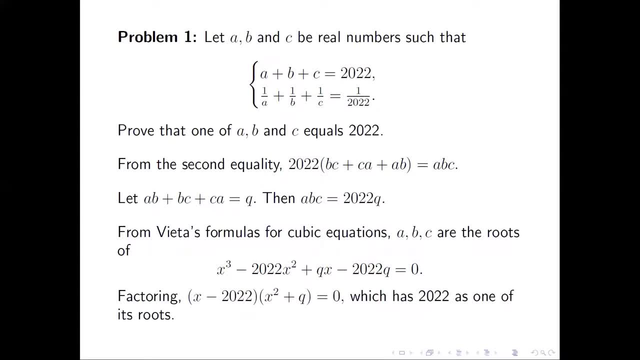 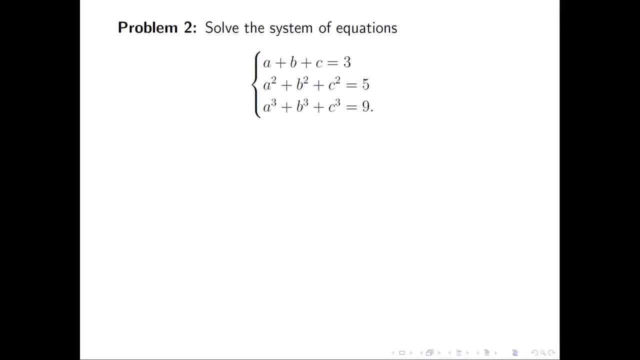 This can be easily factored: X minus 2022 times x, squared plus q equals zero. This always has a root: 2022.. Problem number two: All the equations are cyclic. To apply Vieta's formulas, we need three coefficients. 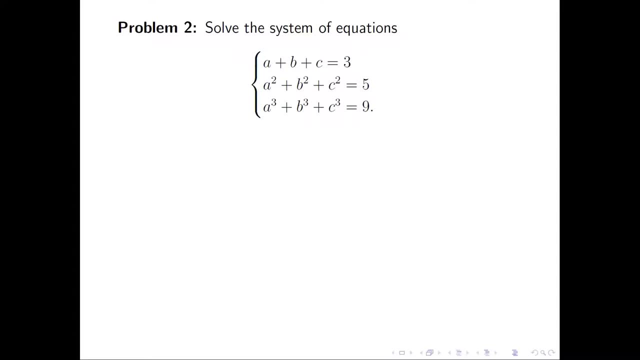 First, a plus b plus c, which we already have, is a three. So we need to calculate the other two coefficients, a b plus b, c plus c. a and a b, c, We square the first equation, a plus b plus c squared. 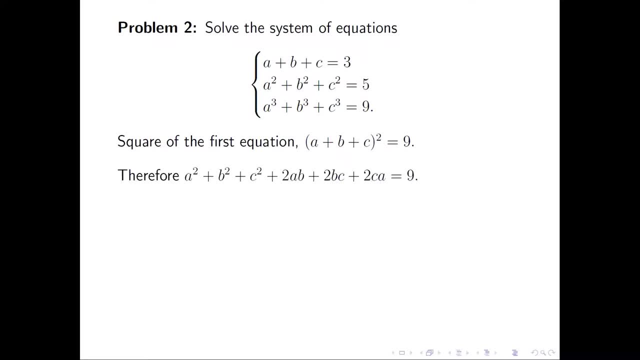 plus c squared plus c squared plus 2ab plus 2b c plus 2c a equals nine. Expanded, we have a squared plus b squared plus c squared plus 2ab plus 2b c plus 2c a equals nine. 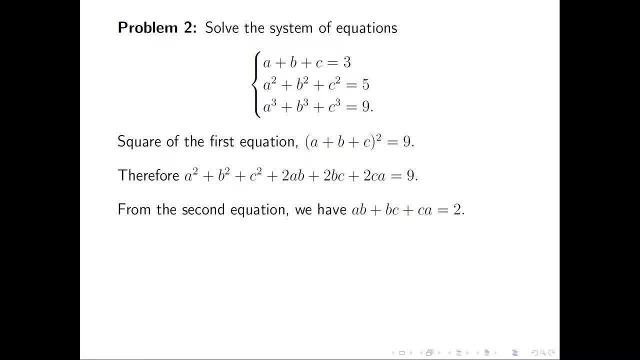 And the sum of the first three terms is five. Therefore, a b plus b, c plus c, a equals two. This is the second coefficient. The third one is slightly tricky. We multiply the first two equations: a plus b plus c, times a squared plus b squared. 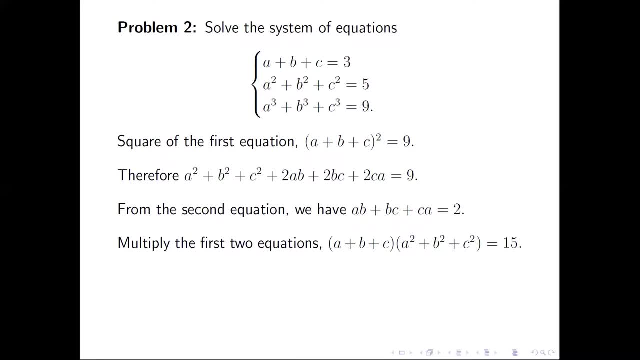 plus c squared equals three times five. Expand the left-hand side: Three terms times three terms. we have nine terms expanded. Of course. the first three terms are a cubed plus b cubed plus c cubed. For the right six terms, we can separate them into three groups. 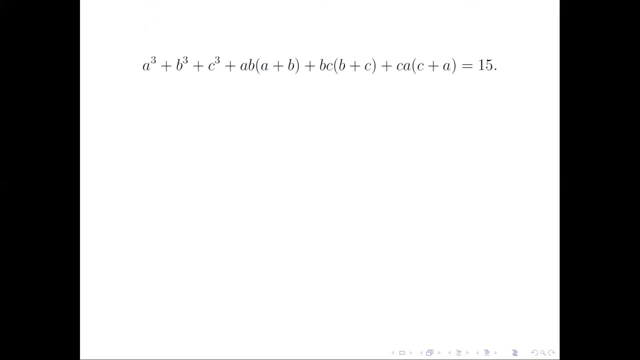 This equation can be further simplified by substitution. We know the sum of the first three terms is 9.. We also know a plus b plus c is 3.. So a plus b plus c is 9.. So a plus b plus c is 3.. 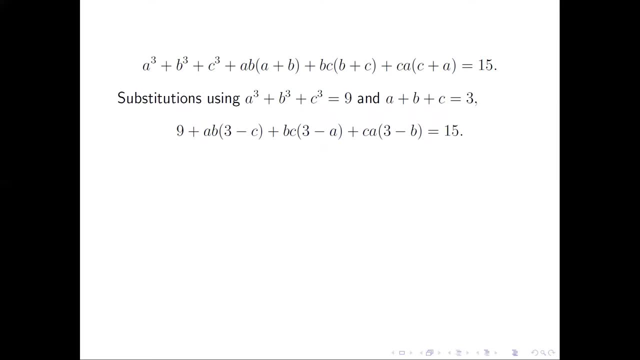 So a plus b plus c is 4.. So a plus b plus c is 5.. b is 3 minus c, b plus c is 3 minus a and c plus a is 3 minus b. Clean it up: We have 3 times ab plus bc plus ca minus 3 times abc equals 15 minus 9.. 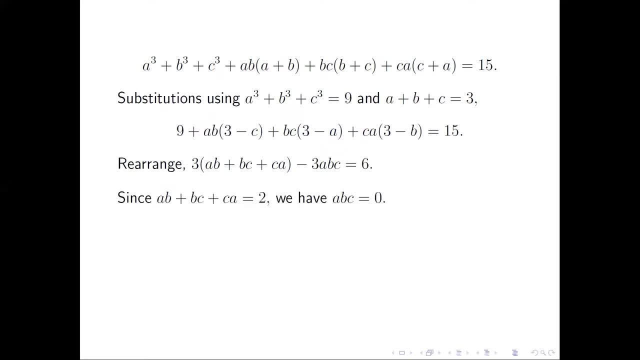 As we just calculated, ab plus bc plus ca equals 2.. Plug it in. we have abc equals 0.. This is the last coefficient, the constant By Vieta's formula. ab and c are the rules of the cubic equation: x cubed minus 3x, squared plus 2x minus 0, equals 0.. 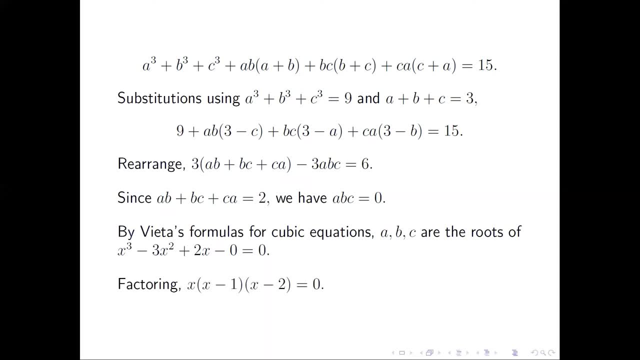 Factor it, We got the solution. abc equals 012 or any permutation. Thank you for watching. Please consider subscribing to my channel. I appreciate your support.